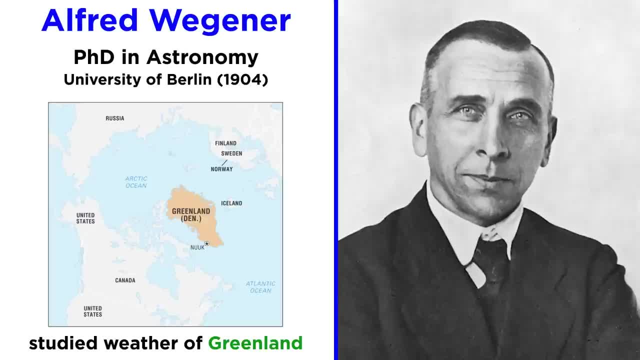 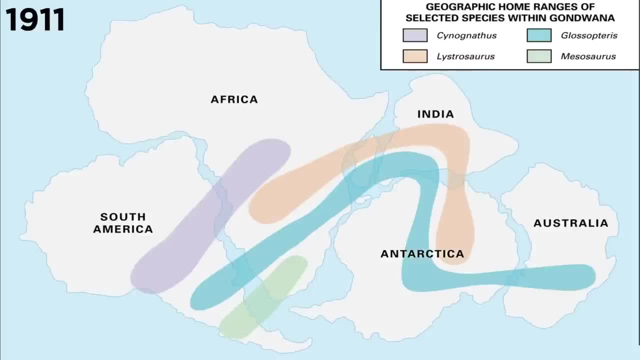 In an odd turn of events, he spent most of his career studying the weather of very cold places like Greenland. In 1911, Dr Wegener came across a paper on the presence of similar Permian-aged fossils in disparate places like South America and Africa or Antarctica, and 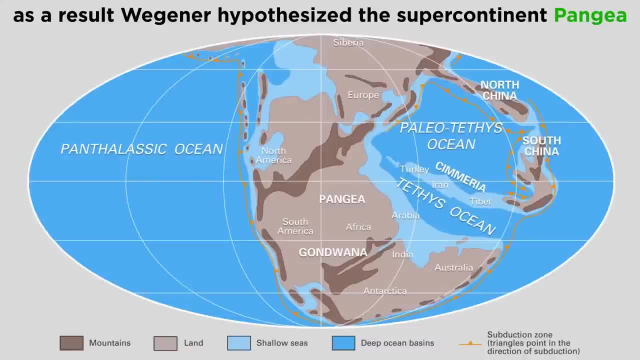 Australia. He concluded that the only way these organisms could have existed together would be if all the continents had been joined together into one huge, huge supercontinent, which he named Pangea. Unfortunately, Dr Wegener died of overexertion. 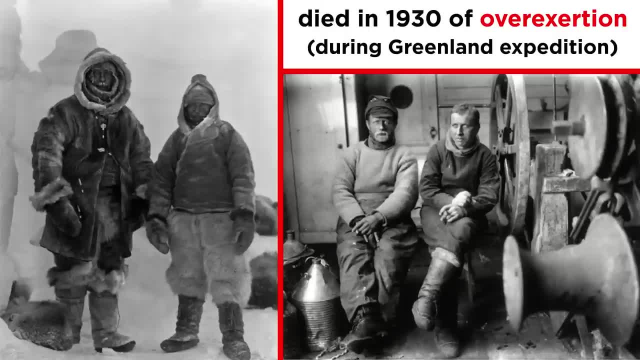 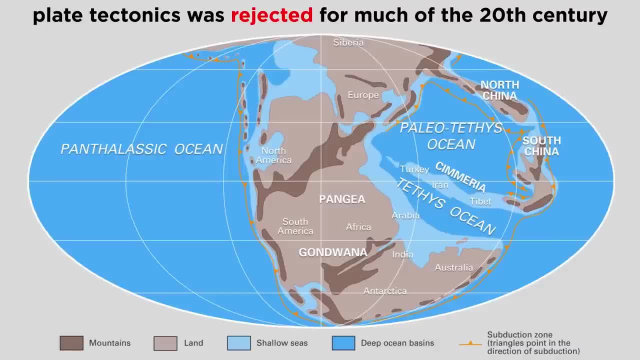 during one of his Greenland expeditions, before he could substantiate Pangea's existence. In fact, the idea of Pangea and the theory of plate tectonics that it relied upon was resoundingly rejected throughout much of the 20th century. 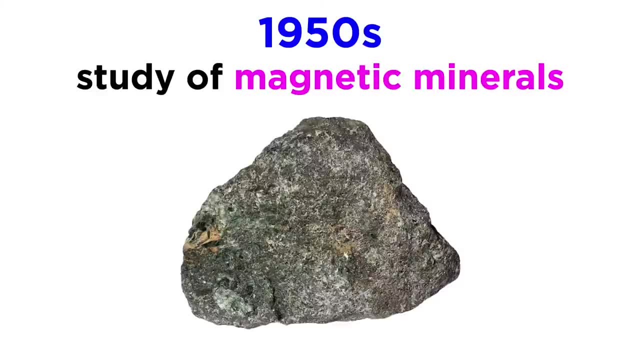 Further evidence for plate tectonics came in the 1950s during the study of magnetic minerals in rocks. When a new technology was introduced, it was known as the plate tectonics. The plate tectonics were a technical term that was used to describe the magnetic field around the Earth. 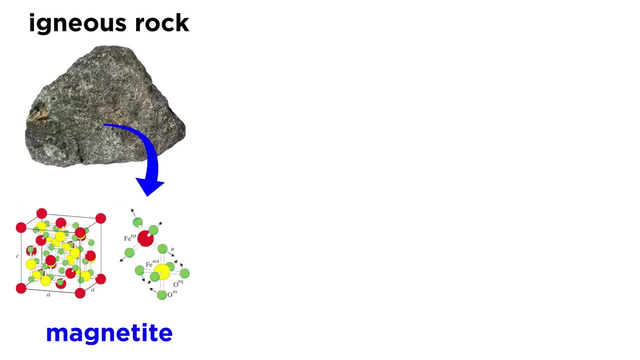 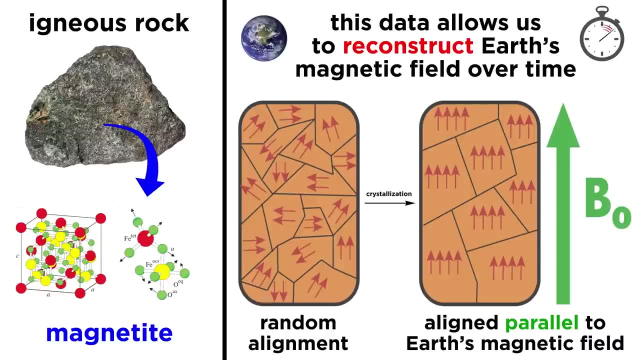 When an igneous rock crystallizes, tiny needles of the mineral magnetite align themselves parallel to Earth's magnetic field lines, and studying the orientation of these magnetic fossils, so to speak, makes it possible to reconstruct Earth's magnetic field over time. Now Earth's magnetic field does somewhat drift around the poles. 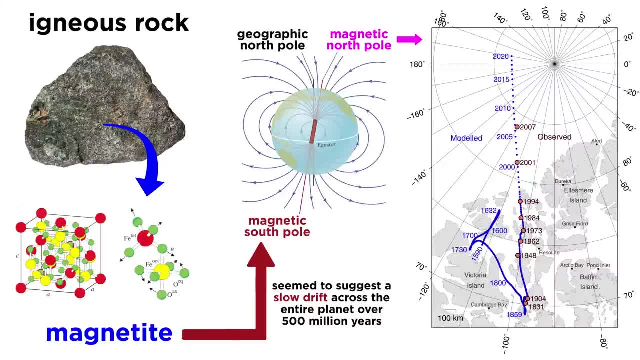 but the study of these magnetic rocks seemed to indicate that over the past 500 million years Earth's southmost magnetic field will also drift around its poles. The magnetic field is, of course, magnetic pole drifted from the Northern Hemisphere through the equator and to its present location. 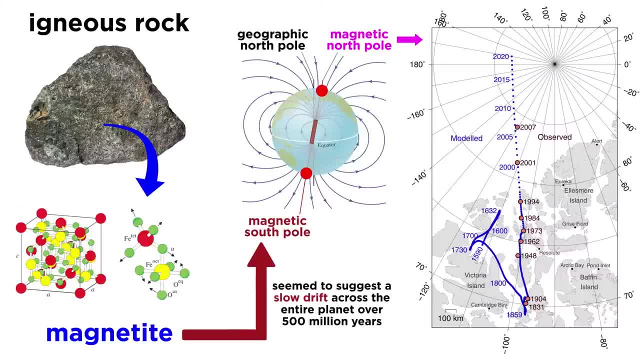 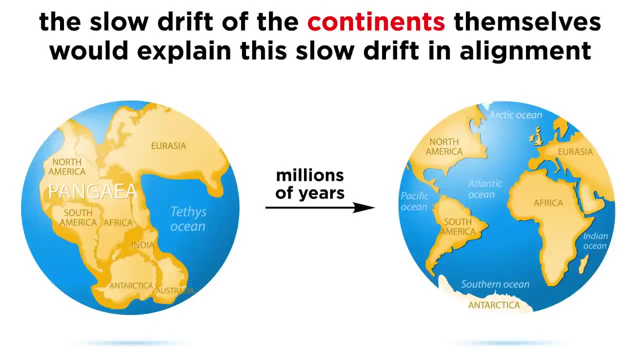 over the geographic South Pole, but the magnetic poles must be located near the geographic poles because the magnetic field is strongly related to Earth's rotation. Therefore, this observation could only be explained by the movement of the continents themselves over a semi-stationary field. 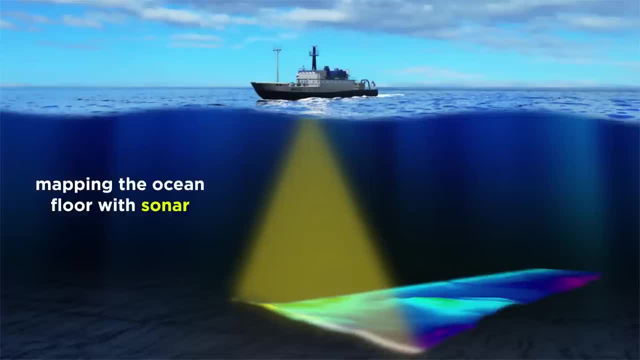 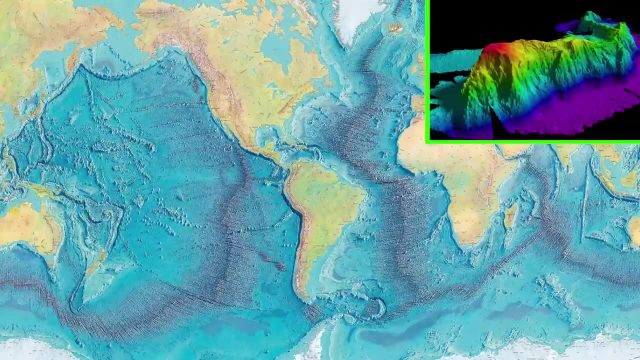 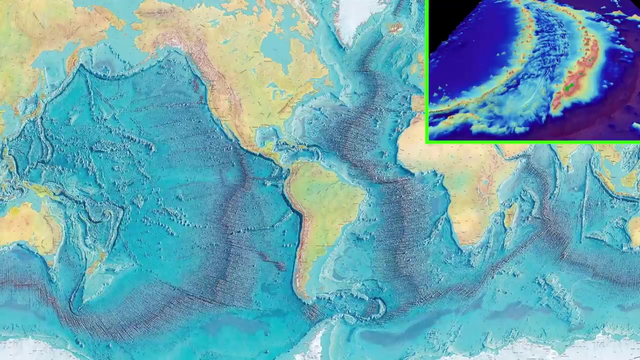 Throughout World War, Two geologists used sonar to map the ocean floor and were shocked by the topography they discovered. The ocean floor wasn't a flat plain, but rather was full of mountain ridges, with perpendicular fractures, deep trenches and long chains of underwater volcanoes. 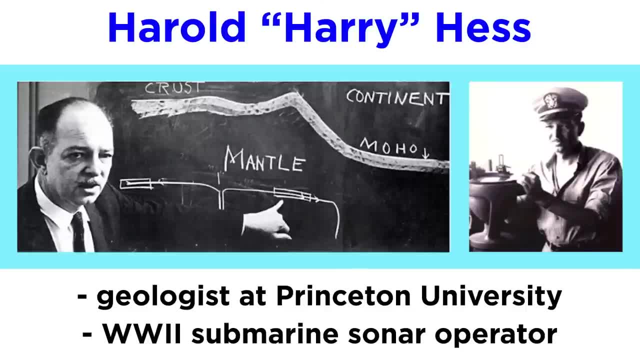 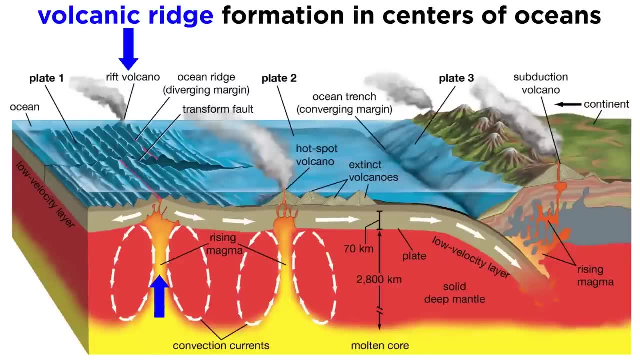 Based on this data, Harold Hess, a geologist from Princeton University and former World War Two submarine sonar operator, proposed a theory for how continents might move. Hess postulated that the linear volcanic ridges at the centers of oceans were caused by areas. 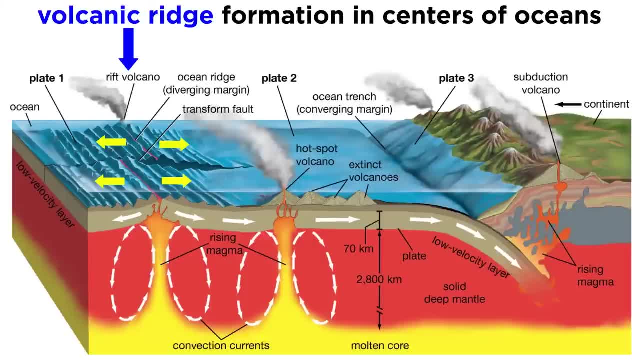 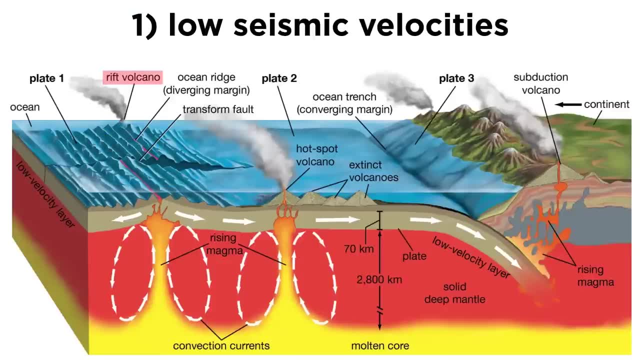 of convection-driven hot rising mantle that solidified and spread out laterally to create new oceanic crust. Evidence for this included low seismic velocities, the presence of volcanoes and high heat flow from the mantle at these mid-ocean ridges. 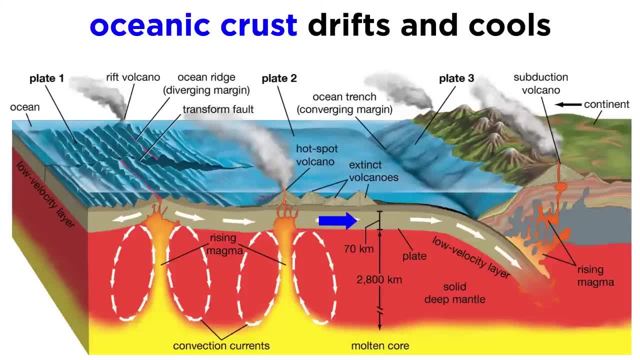 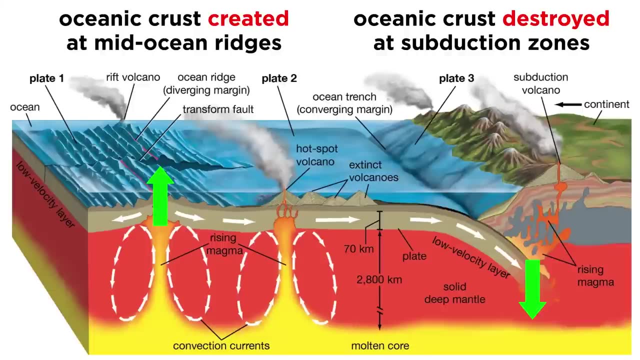 Once formed, oceanic crust moves away from the ridge, Cooling and becoming more dense with age, until it eventually sinks back into the mantle at deep sea trenches. According to Hess's theory, the simultaneous creation of oceanic crust at mid-ocean ridges. 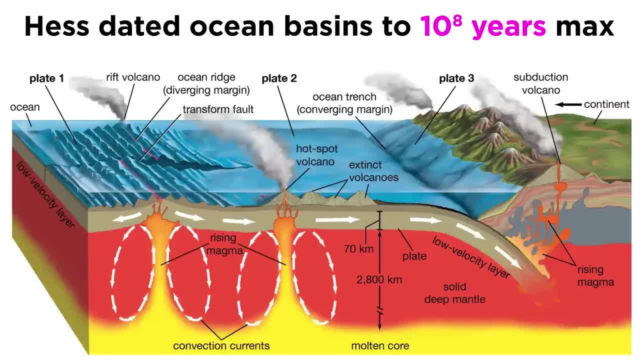 and its destruction at subduction zones would limit the age of the world's ocean basins to a few hundred million years, which agreed with the relatively thin layer of pelagic sediment on the seafloor. Though the evidence described so far may not be accurate, the theory is that oceanic 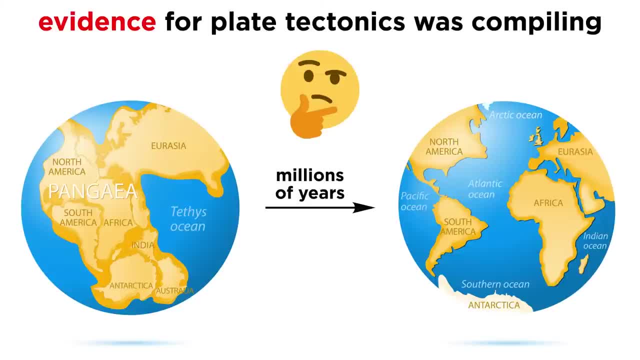 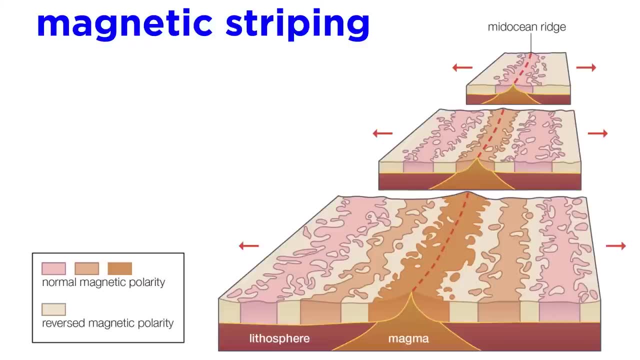 crusts have been formed over a period of time. The discovery of magnetic striping of the seafloor may seem convincing. it was still only circumstantial at the time, but not for long. The smoking gun would eventually come from the discovery of magnetic striping of the 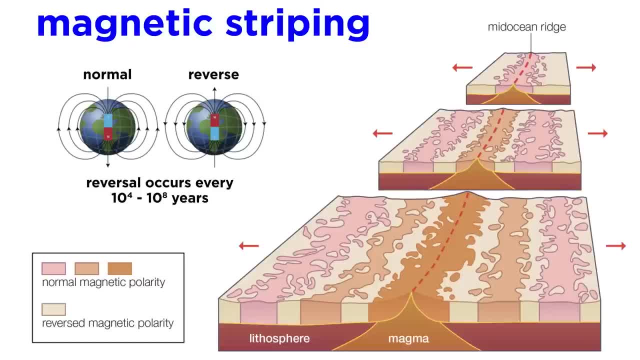 seafloor. Prior to this discovery, paleomagnetism had been extensively studied in terrestrial rocks and it was well known that the Earth's magnetic field periodically reversed. The current configuration of the magnetic field is said to be normal polarity and the 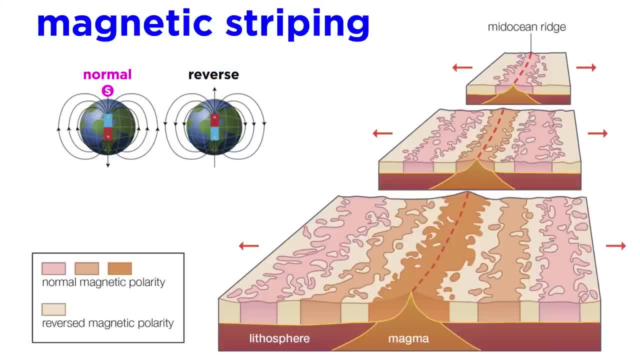 flipped polarity is called polarity. Paradoxically, the magnetic pole located at the North Pole today is actually the magnetic South Pole, since magnetic field lines always point from the north to the south pole of a magnet. At any rate, if Hess was right, the magnetic striping along the seafloor would be mirrored. 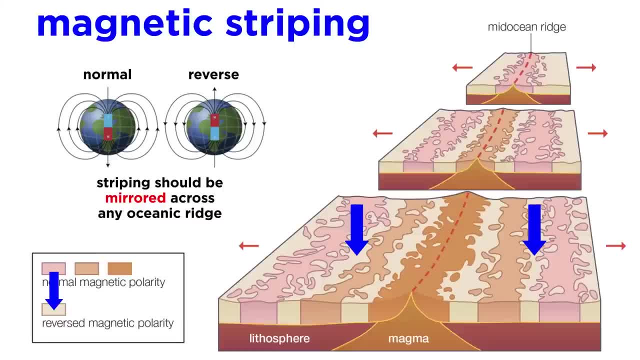 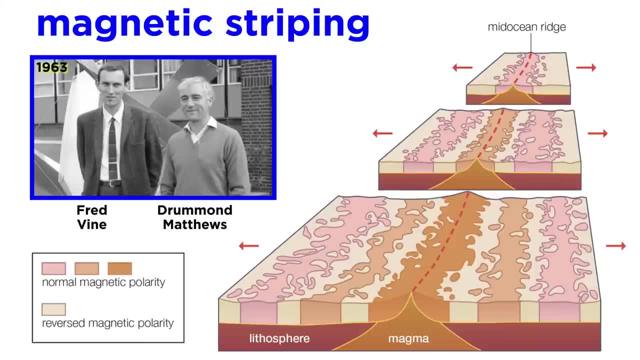 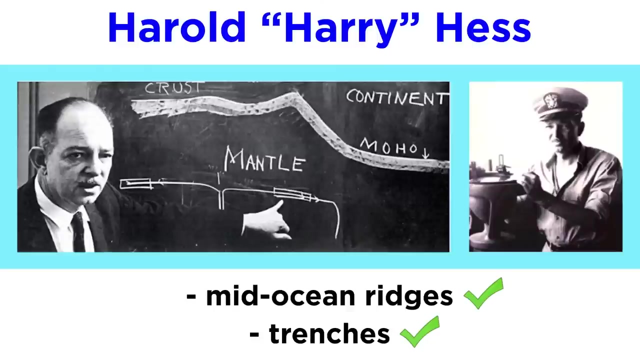 across the ridge and correspond to the already known record of magnetic reversals. And in 1963, Fred Vine and his PhD advisor Drummond Matthews provided the evidence leading to the wide acceptance of the theory of plate tectonics. While Dr Hess' work explained the formation of mid-ocean ridges and trenches, there were 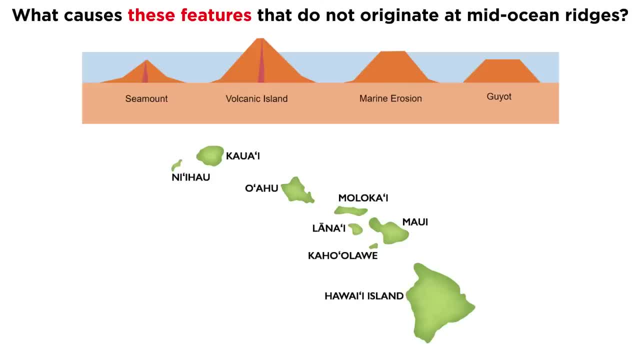 still two pesky questions left unexplained. First, how were seamounts formed like the Hawaiian Islands? And second, what created long perpendicular fractures in the seafloor? And the second question is: what is the reaction to the big-bottomed seafloor? The first was the reaction to the construction of the mid-ocean ridge and the second was the reaction to the expansion of the seafloor. The second was the reaction to the expansion of the seafloor And the third was the reaction to the expansion of the seafloor. 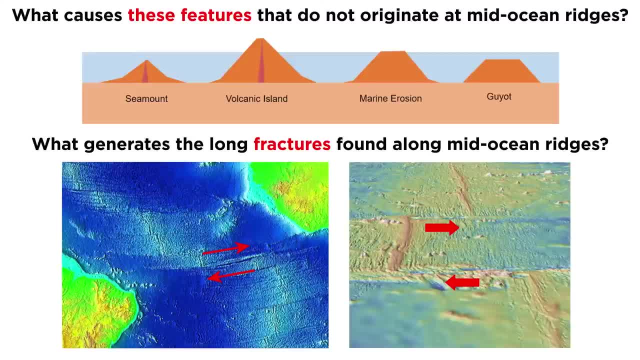 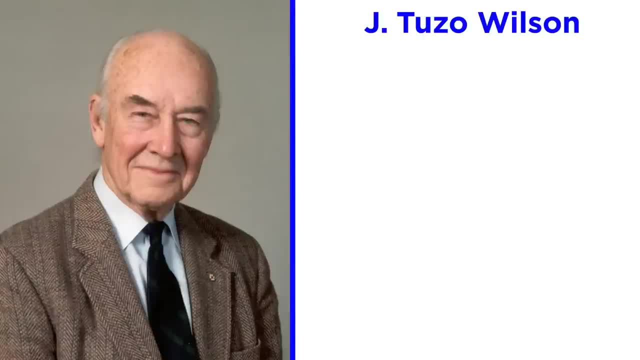 The third was the reaction to the expansion of the seafloor along mid-ocean ridges, as exemplified along the South Atlantic Ridge. In 1963, Canadian geologist J Tuzo Wilson figured out the answer. He proposed that 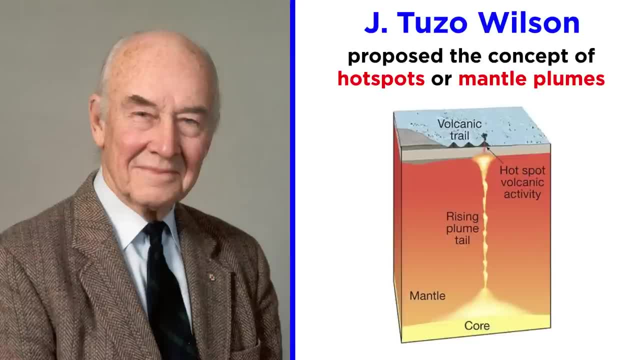 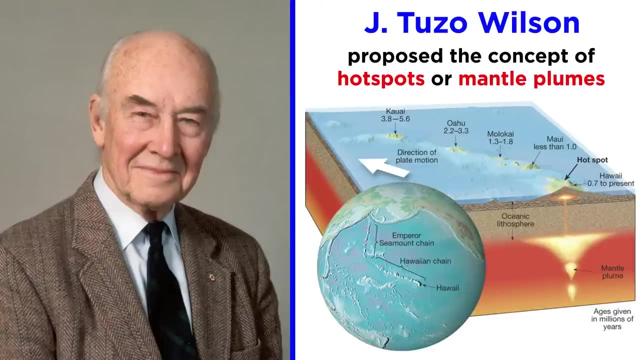 seamounts were formed due to volcanism induced by a cylindrical stationary area of hot rising mantle called hotspots, or, more specifically, mantle plumes. Using the Hawaiian Islands and the Emperor Seamounts as an example, Dr Wilson observed that the alignment of the island chains 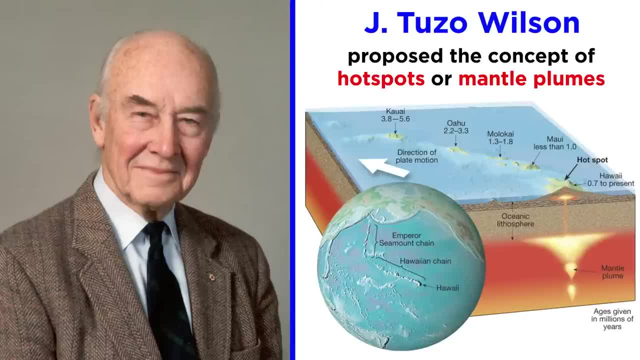 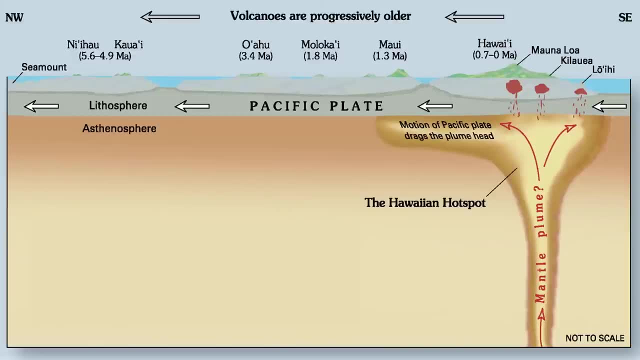 followed the motion of the Pacific Plate, which led him to develop the following understanding of seamounts: At some point in time, a mantle plume forms beneath an area of the crust which leads to the initiation of volcanism. Then, over millions of years, the plate moves. 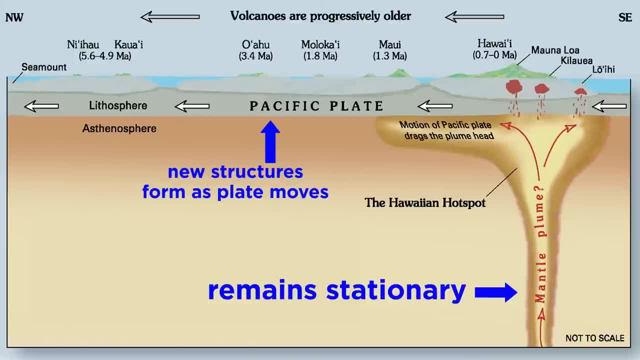 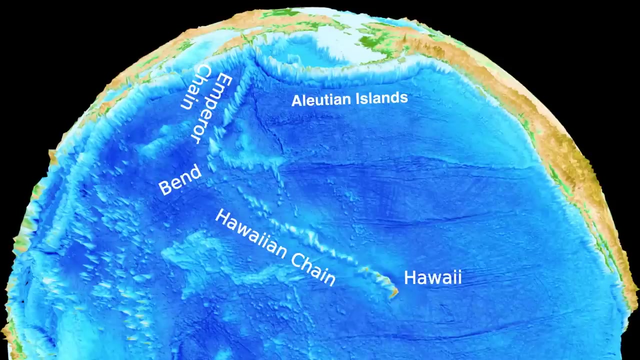 steadily over the stationary mantle plume, leaving a long trail of inactive volcanic islands. As an area of the crust moves off the hotspot, volcanism shuts off and the seamount begins to be slowly eroded by the sea. When looking at a satellite image of the Pacific Ocean, 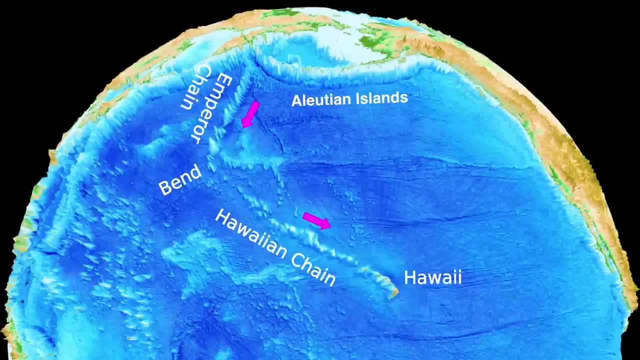 you can see a chain of increasingly eroded seamounts extending all the way from Hawaii, which is currently beneath the plume, to the Aleutians. This is a precise recording of the Pacific Plate's motion over the past 65 million years, called a hotspot track. 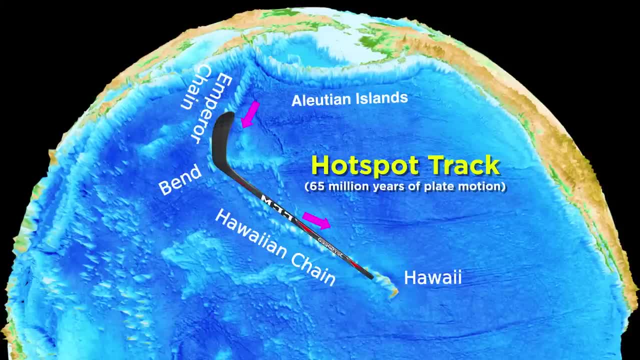 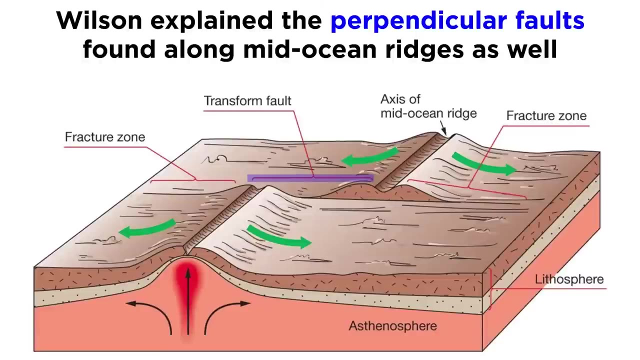 Interestingly, it is not linear, but is shaped like a hockey stick, which beautifully illustrates a sudden change in plate motion that occurred around 40 million years ago. Two years after proposing mantle plumes, Dr Wilson suggested an explanation for the perpendicular faults along mid-ocean ridges: Mid-ocean ridges don't form.